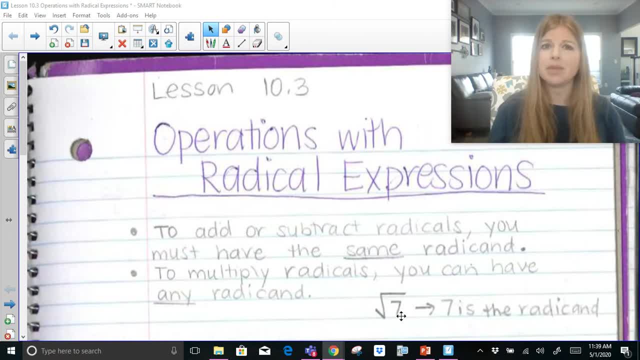 You could do 2x plus 3x and get 5x, but you can't do 2x plus 3y. They're not like terms. The same thing happens with radicals: You have to have the same radicand in order to actually add them. 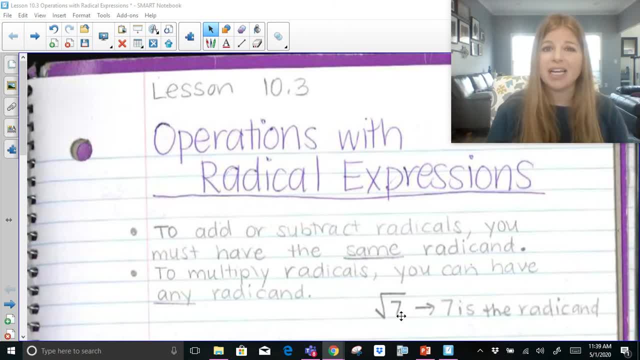 To multiply radicals. you can have anything you want, Kind of like you can do 2x times 3y and get 6xy. So radicals are going to follow that same procedure. So the different operations that we're going to take a look at, we're going to add and subtract like radicands. 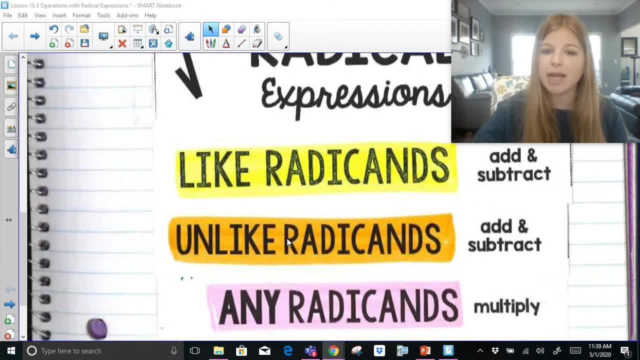 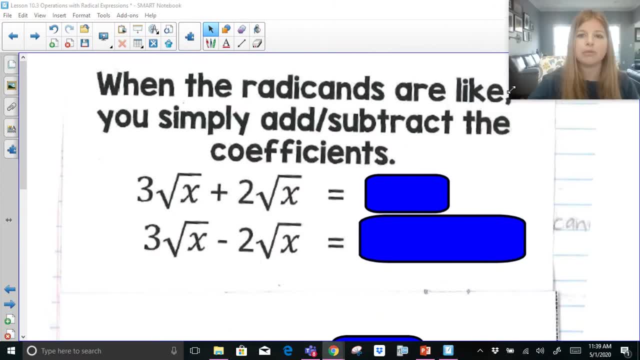 So ones that are the same. We're going to learn how to add and subtract, unlike radicands, And we're going to learn how to multiply with any radicand, It does not matter. All right, so it says here: when the radicands are like you, simply add or subtract the coefficients. 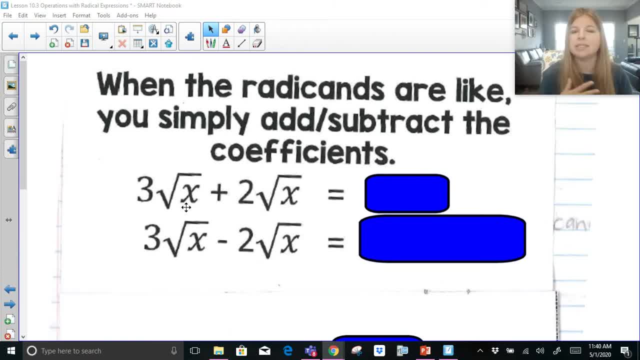 So if I have 3 radical x, You're going to hear me guys say radical x or root x. They mean the same thing: 3 radical x plus 2 radical x. That would mean I have 5 radical x. Just like combining, like terms. 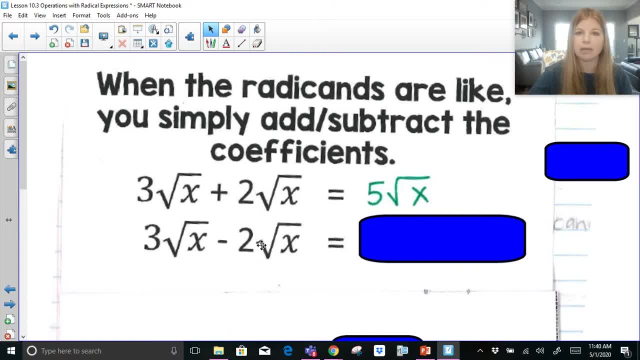 Same thing with the next one. If I have 3 radical x minus 2 radical x, Well, 3 minus 2 is 1.. So that would just simply be 1 radical x, which is just radical x. So notice, I didn't do any operations with the radicand, the variable, that's the value that's under the radical sign. 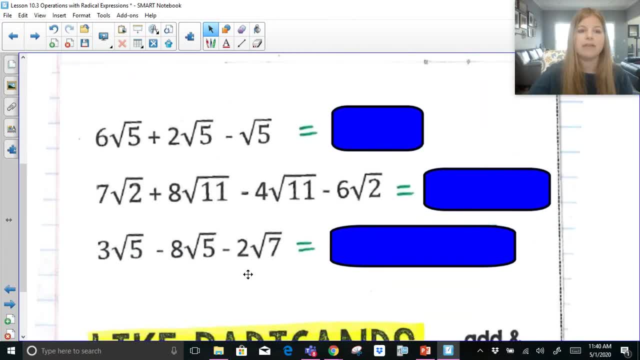 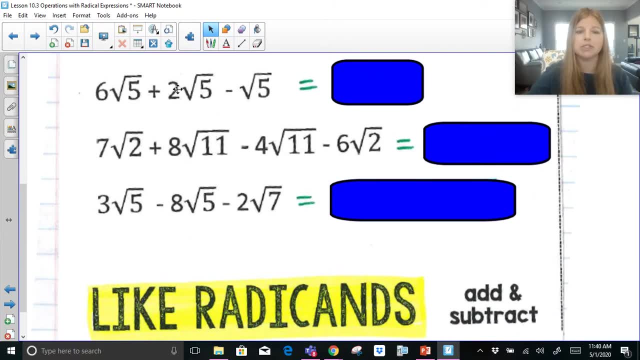 I just took care Of the coefficients. So now if I have 6 radical 5 plus 2 radical 5 minus radical 5. I'm really dealing with again my coefficient. So 6 plus 2 is 8.. 8 minus 1 is 7.. 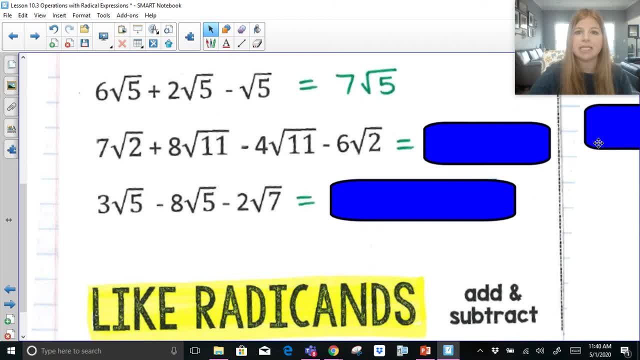 So this is 7 radical 5.. Notice, the radical 5 stays. I didn't change it or touch it. Now this one: 7 radical 2 plus 8 radical 11 minus 4 radical 11 minus 6 radical 2.. 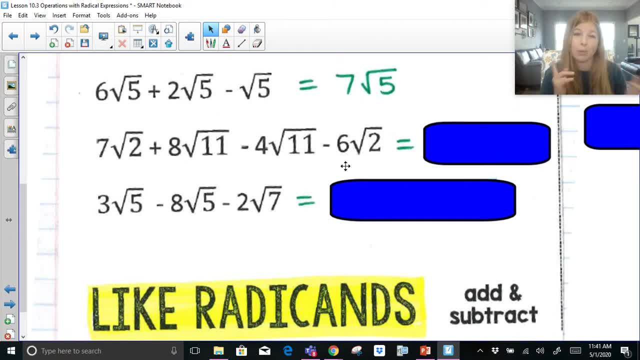 This is like when you're combining like terms and some of them are x's and some of them are y's. This is like when you're combining like terms and some of them are x's and some of them are y's And you have to match up the right ones. 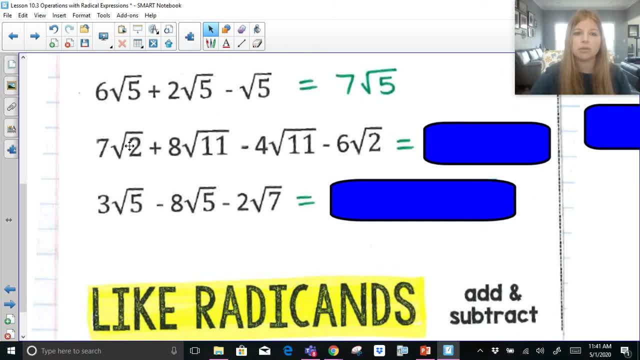 Same idea here. So 7 radical 2 goes along with a negative 6 radical 2.. So 7 minus 6 is 1.. So that would just give us radical 2.. Then I'm going to look at my radical 11s. 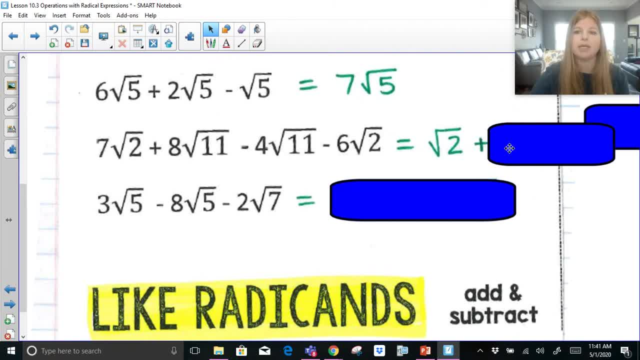 8 radical 11 minus 4 radical 11 would be 4 radical 11 and a positive 1. Now you can write radical 2 plus 4 radical 11.. You can also have them in reverse order: 4 radical 11 plus radical 2.. 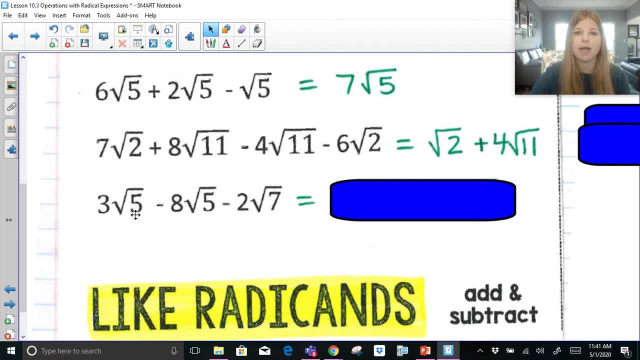 Either answer is fine. The last one here: 3 radical 5 minus 8 radical 5 minus 2 radical 7.. Now I only have three terms here and two of them have the same radicand. So 3 radical 5 minus 8 radical 5 is negative. 5 radical 5.. 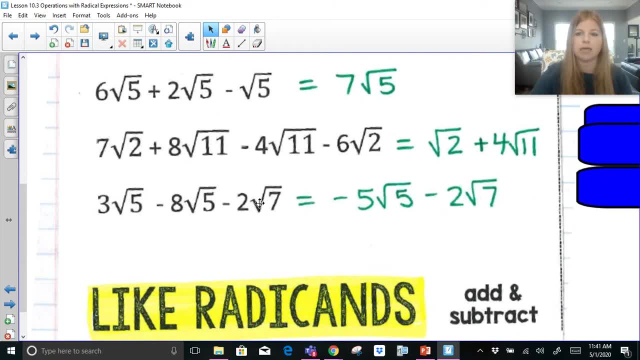 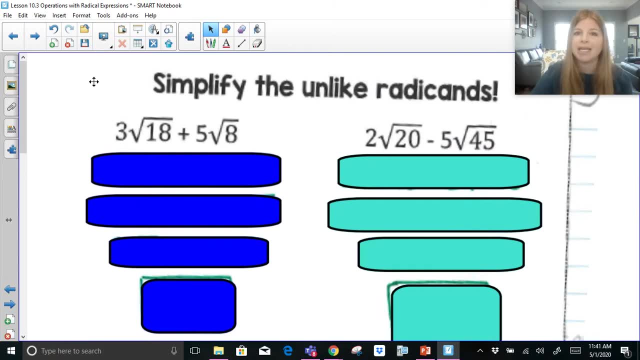 And this negative 2 radical 7 just stays minus 2 radical 7.. It has nothing to combine with. The next thing we're going to look at is when we have to add or subtract. but the radicands are not like. So here we have. 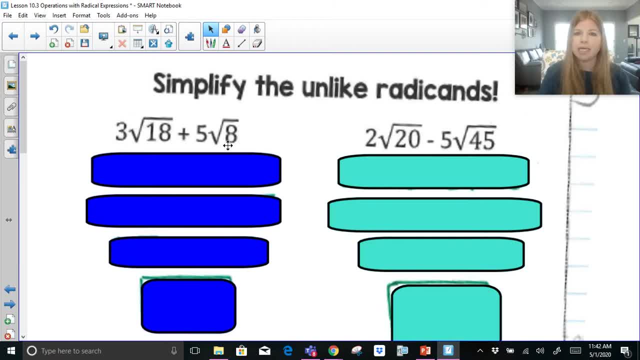 3 radical 18 plus 5 radical 8, and from our last part of our lesson We just saw that, hey, we can't add these. but something we know how to do is we know how to simplify radicals. Now look at radical 18.. 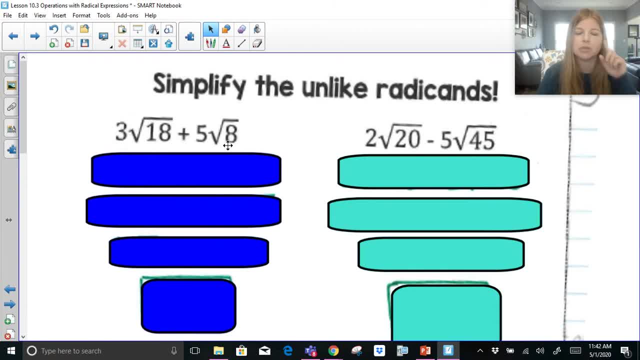 You can break apart radical 18.. Think about it. What's the biggest perfect square that goes into 18? It's 9.. So this really becomes 3 and radical 18 breaks up into radical 9, radical 2.. Remember the process. you find the biggest perfect square that divides into: 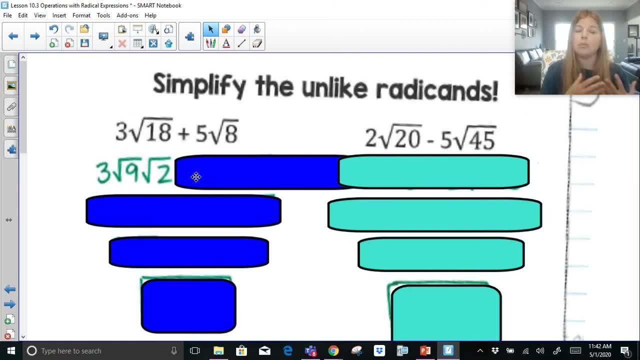 18, which is 9. you keep that in front 9 times What is 18: 2, so it breaks up into radical 9, radical 2 plus 5, nothing about 8.. Is there a perfect square that goes into 8?? 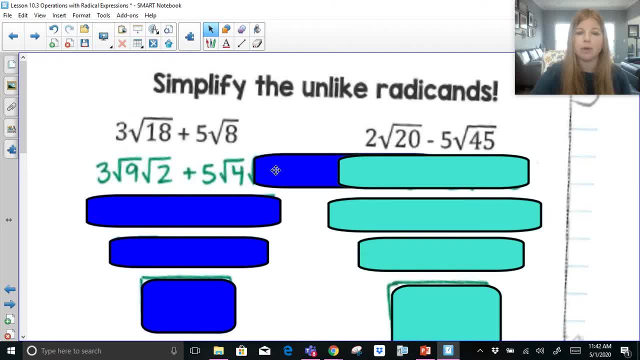 It's 4, so radical 8 gets broken up into radical 4, radical 2: always put the perfect square first, guys. So now let's simplify what we can. this becomes 3 times when we know the square root of 9.. It's 3. bring down the radical 2.. 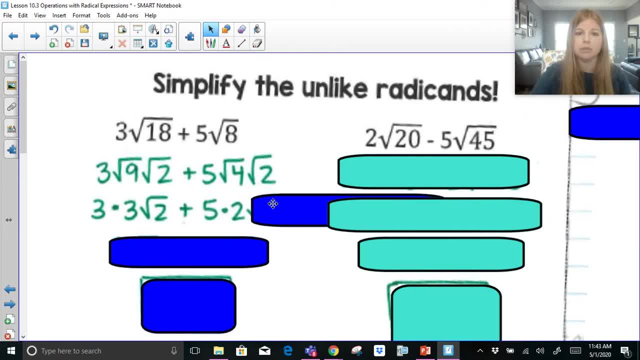 Plus 5 times, We know the square root of 4.. It's 2 radical 2.. I hope you see where this is about to go. 3 times 3 is 9.. So I've got 9 radical 2 plus 5 times 2 is 10.. 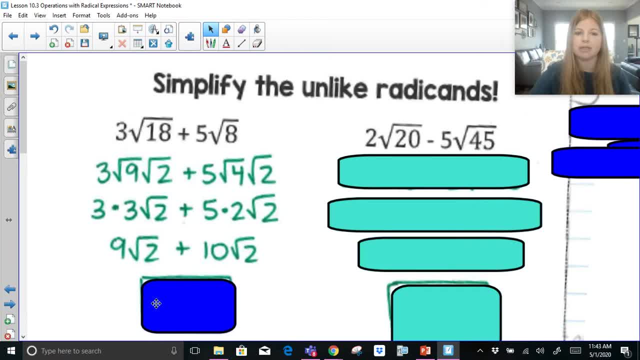 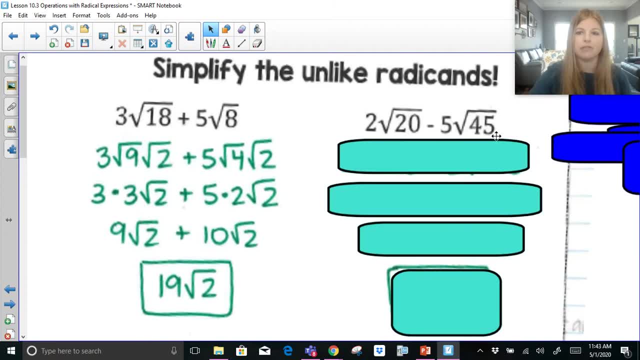 So it's 10 radical 2, 9 radical 2 plus 10 radical 2 is 19 radical 2. pretty good, Let's try the next one: 2 radical 20 minus 5 radical 45. again, They're unlike radicands. 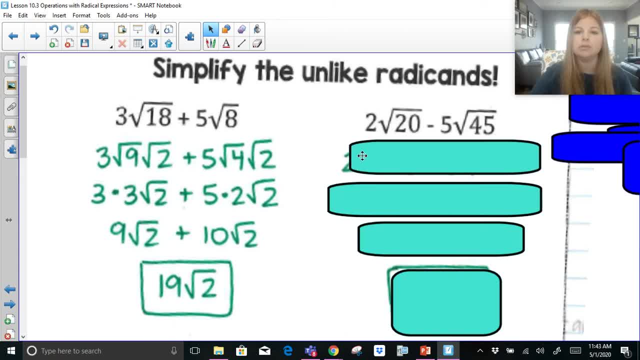 but let's simplify them to see what it brings us. 2: biggest perfect square that goes into 20 is 4.. So it'd be radical 4, radical 5 minus 5 times 45. biggest perfect square that goes into 45 is 9.. 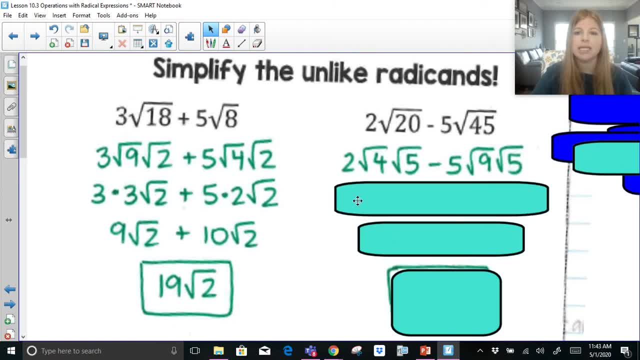 So that's radical 9 radical 5.. This now becomes 2 times 2, because the square root of 4 is 2 radical 5 minus 5 times The square root of 9 is 3 radical 5, which then becomes 4 radical 5 minus 15.. 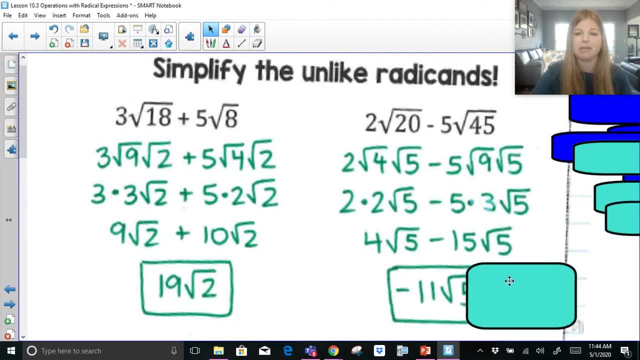 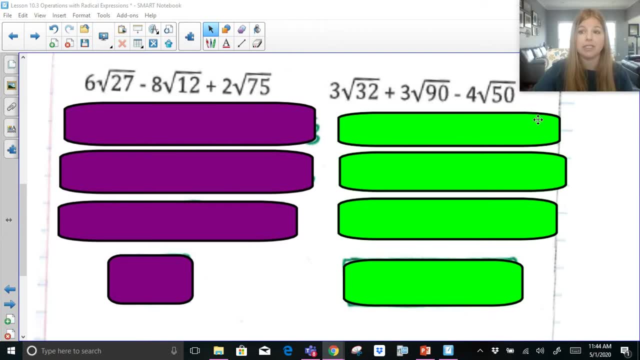 Radical 5: 4 minus 15 is negative 11. radical 5: pretty good, All right next to, if you are feeling adventurous and you think you can do these two on your own. There's three terms instead of two, but the process is the same. 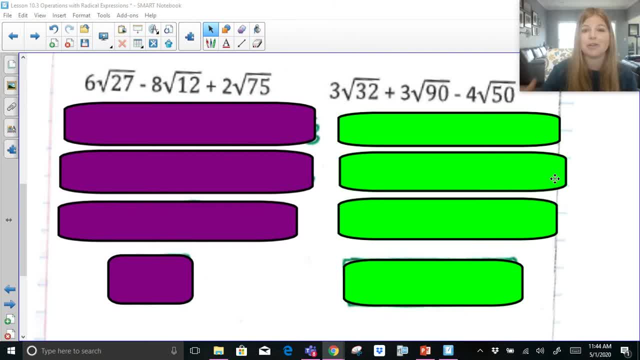 I would press pause right now and then press play after to see how you did otherwise follow along with me. So it's 6 radical 27 becomes 6 radical. 9 radical: 3: biggest perfect square that goes into 27 is 9 minus. 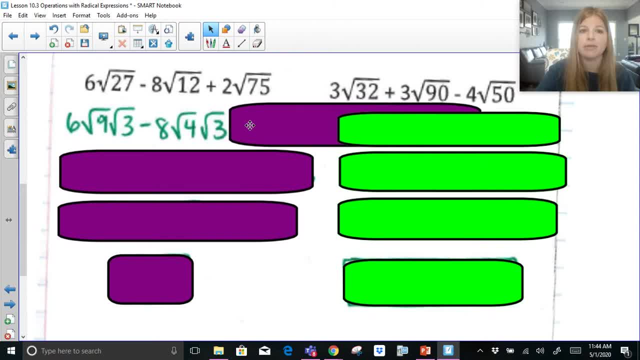 8- 12 breaks up into radical 4: radical 3 plus 2: 75 breaks up into radical 25: radical 3.. This becomes 6 times 3 radical 3 minus 8 times 2 radical 3 plus 2 times 5 radical 3.. 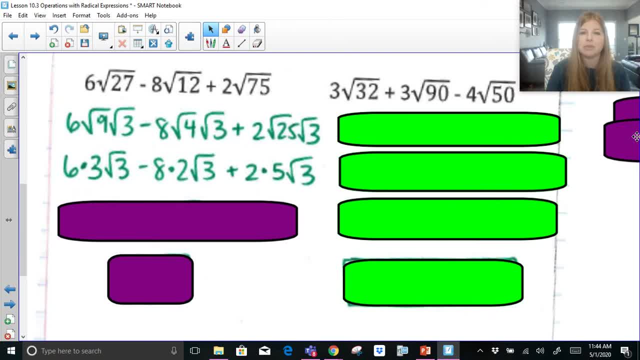 Now, while I'm doing this, I remember a common mistakes. my mistake my students would make is they would look at radical 9 and they wouldn't just write 3, they would write radical 3 and remember the moment You take the square root of a number. 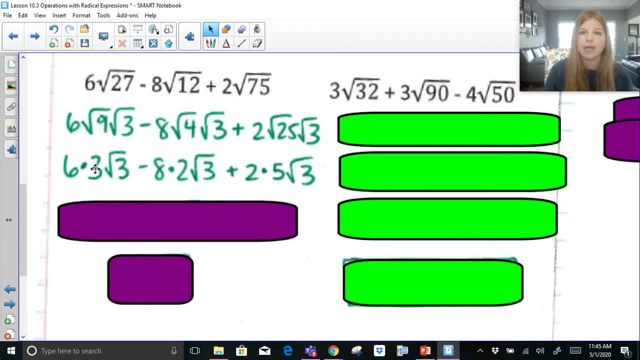 It doesn't need the radical anymore. You wouldn't do that. Like when you took the absolute value of a number, you drop the absolute value bars. It's the same idea. So if you're finding that you are writing more radicals down, you don't need them. 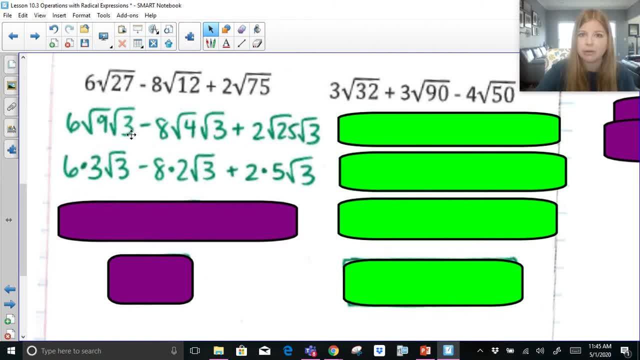 You only leave in the radical what actually you can't simplify like radical 3 is just radical 3.. So now this becomes 18 radical 3 minus 16 radical 3 plus 10 radical 3.. Look at all those radical 3's. we can add up all of our coefficients. 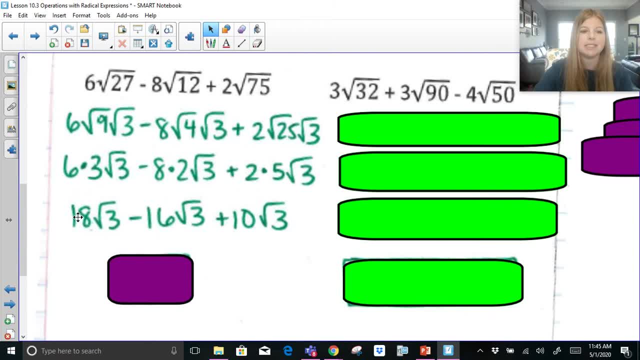 So 18 minus 16.. It's 2. 2 plus 10 would give us 12 radical 3.. Awesome. next one, 3. now radical 32 always tricks people. people think to divide by 4, but 4 is not the biggest perfect square. 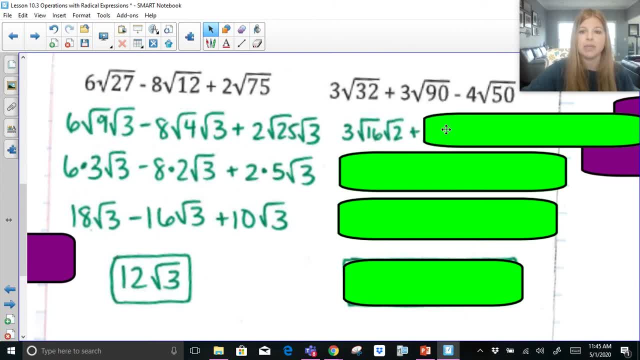 It's actually 16.. So radical 16. radical 2 plus 3: biggest perfect square that goes into 90 is 9.. So radical 9. radical 10 minus 4. biggest perfect square that goes into 50 is 25.. So radical 25.. 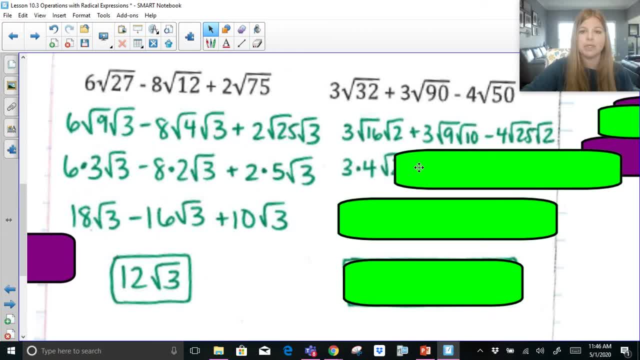 Radical 2.. This becomes 3 times 4 radical 2 plus 3 times 3 radical 10 minus 4 times 5 radical 2.. So now I've got: 3 times 4 is 12 radical 2 plus 3 times 3 is 9 radical 10 minus 4 times 5 is minus 20 radical 2.. 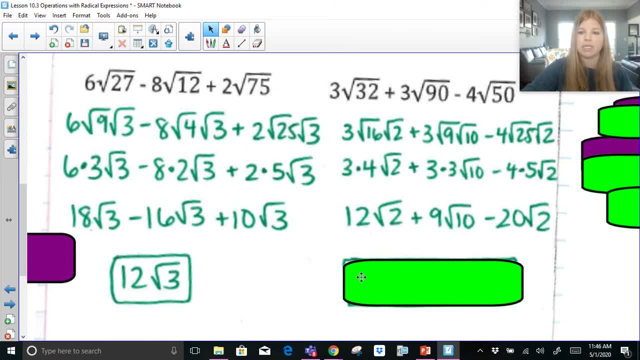 All I have are my radical 2's that are alike. So 12 minus 20 is negative, 8 radical 2 plus 9 radical 10.. And, like I mentioned before, you can reverse the order. You can have it say 9 radical 10 minus 8 radical 2.. 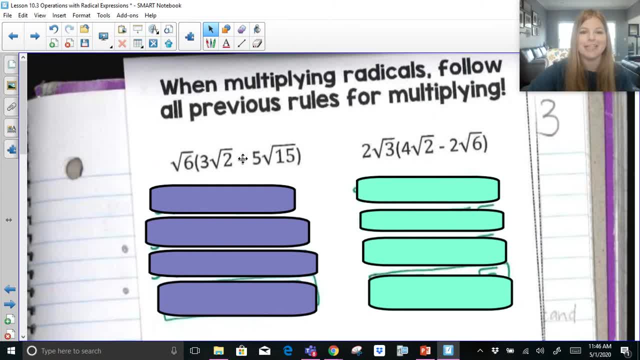 The last tab for this: multiplying. Sorry, my screen is a little crooked here. We follow all previous rules for multiplying. So we had a previous lesson where we're talking about how to multiply radicals and what to do after. So here what should kind of scream out to you is that we have the distributive property going on. 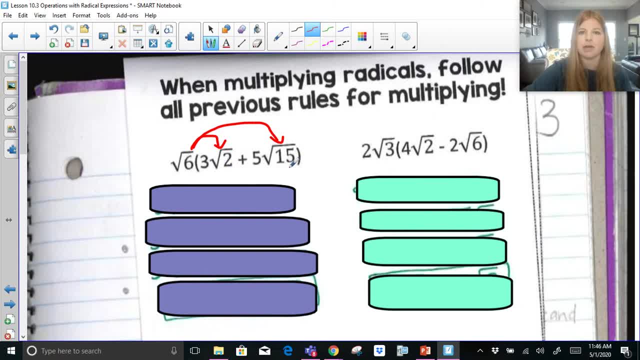 Okay, radical 6 is going to get multiplied by 3- radical 2 plus 5- radical 15.. This here, 2 radical 3- is going to get multiplied by 4- radical 2.. And then it's going to get multiplied by a negative: 2- radical 6.. 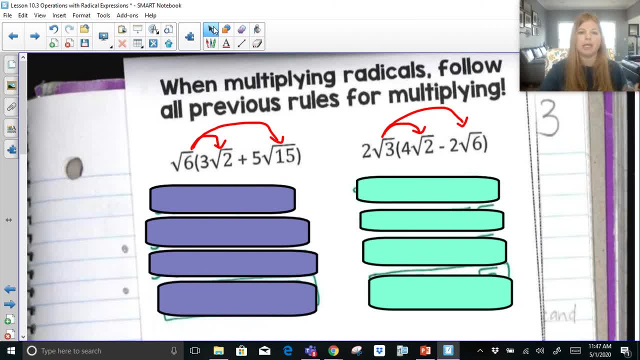 And you don't need the same radicals to multiply, You just multiply as normal. So, 6 radical 6 times 3- radical 2.. Okay, radical 6 times 3- radical 2.. There's really a 1 in front of the radical 6.. 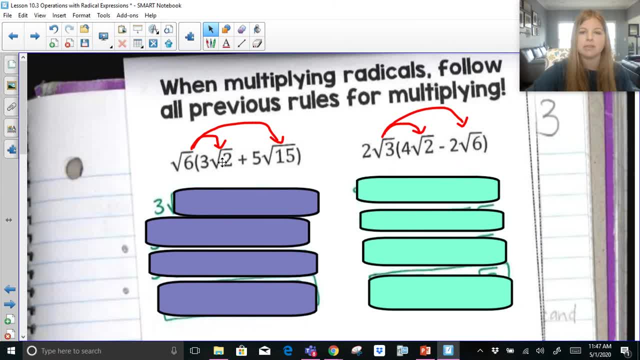 So 1 times 3 is 3.. Radical 6 times radical 2 is radical- My mouse first. Radical 6 times radical 2 is radical 12.. Now I distribute here: Radical 6 times 5, radical 15.. 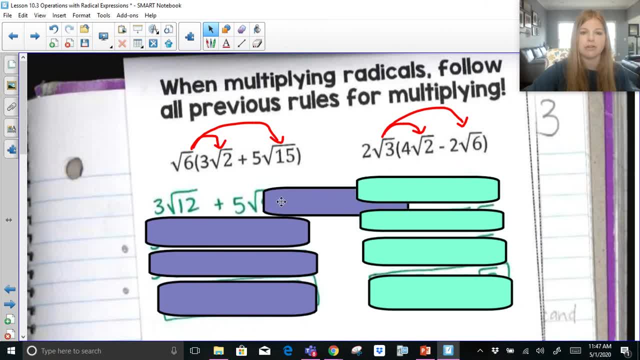 So 1 times 5 is 5.. Radical 6 times radical 15 is radical 90. Now we know from our previous part of the lesson: If they're not like radicals we can't add them. But let's see if we can break them apart. 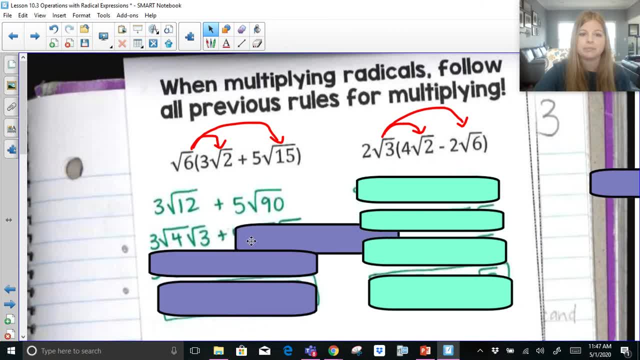 So radical 12 breaks up into radical 4, radical 3.. Plus 5 radical 90 breaks up into radical 9, radical 10.. This becomes 3 times 2 radical 3.. Plus 5 times 3 radical 10.. 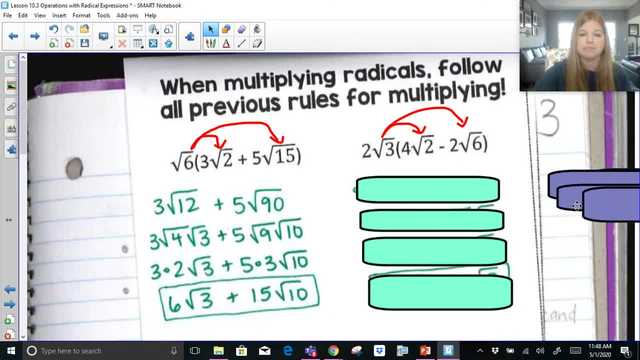 Which becomes 6 radical, 3 plus 15 radical 10.. Can't combine them, Can't do anything else. Next one: 2 times 4 is 8.. Radical 3 times radical: 2 is radical, 6.. 2 times negative: 2 is negative, 4.. 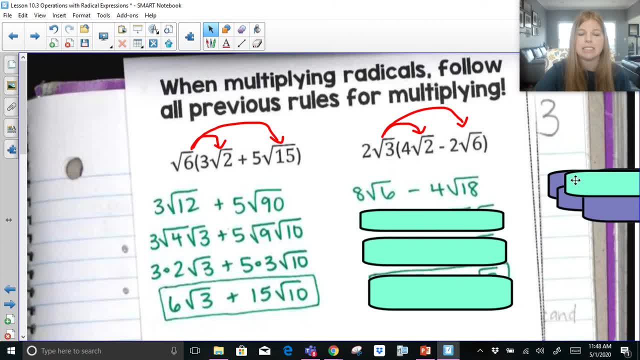 Radical 3 times radical 6 is radical 18.. So 8 radical 6 just hangs out. But I can break apart my radical 18 into radical 9, radical 2. Which becomes 4 times 3 radical 2.. 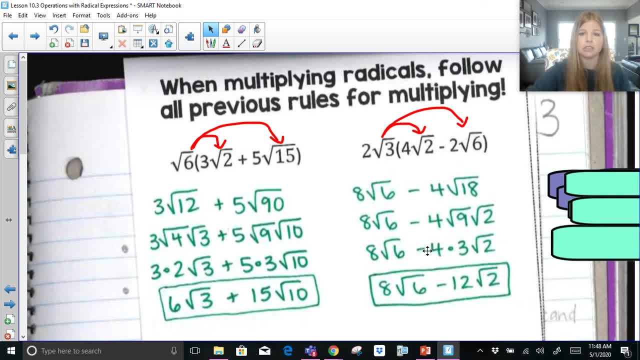 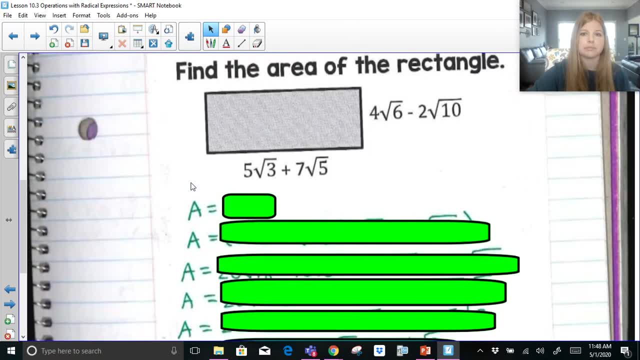 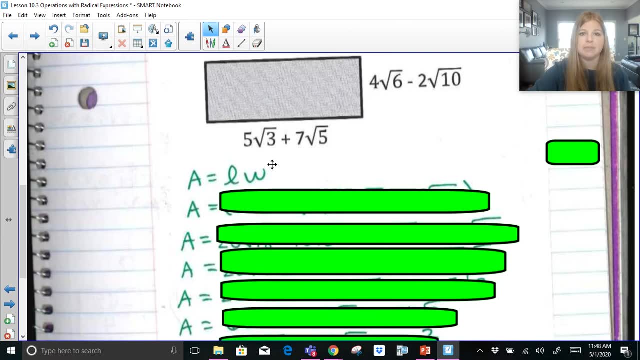 And that's my answer: 8 radical, 6 minus 12 radical 2. Find the area of the rectangle. So area formula, we know, is length times width. So that would mean I have to multiply this expression, Times this expression. Remember when you're multiplying binomials. 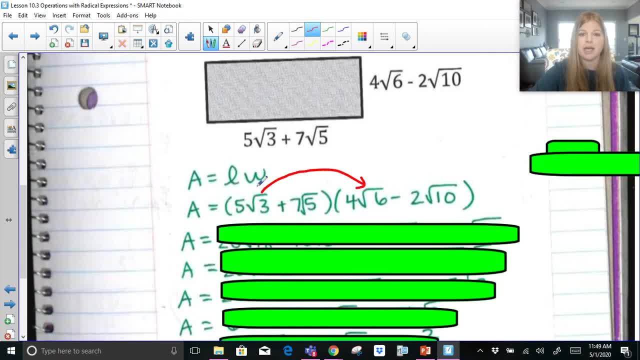 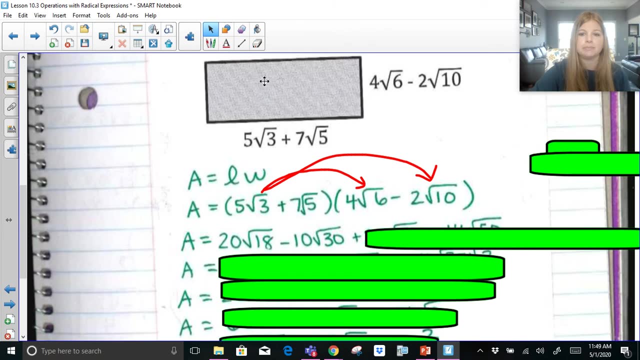 Which is what this kind of comes out to be. We have to distribute the 5 radical 3 first twice. So 5 radical 3 times 4 radical 6 would be 20 radical 18.. 5 radical 3 times negative. 2 radical 10 would be negative. 10 radical 30.. 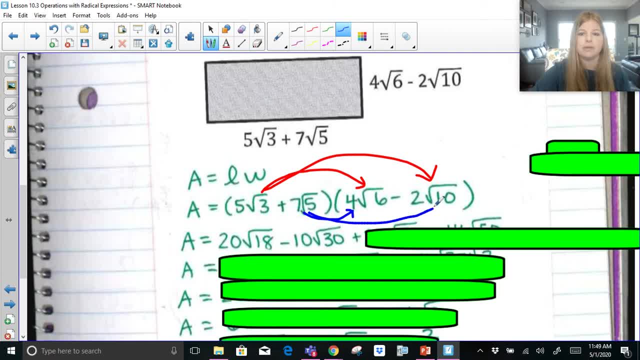 Then we would need to distribute this: 7 radical 5.. So 7 radical 5.. Times 4 radical 6.. So 7 times 4 is 28.. Radical 5 times radical: 6 is radical 30.. 7 times negative: 2 is negative 14.. 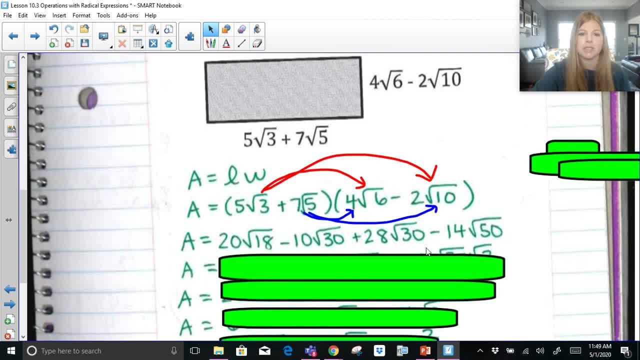 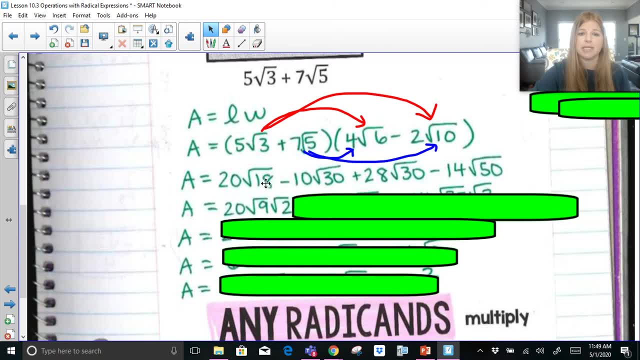 Radical 5 times radical 10 is radical 15.. All right, So now 20 radical 18 becomes 20 radical, 9 radical 2. We can break that apart, Can't break apart radical 30s. But look.